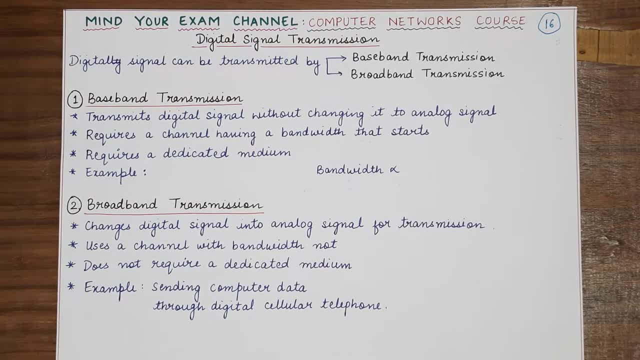 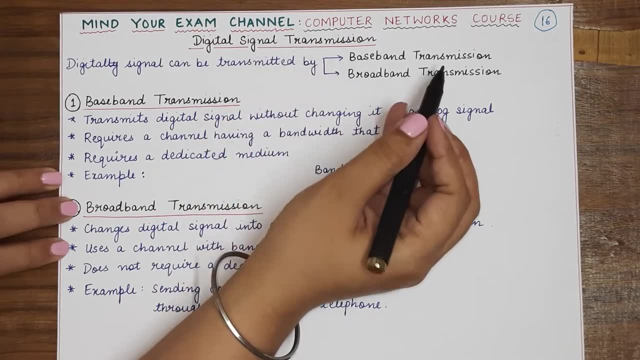 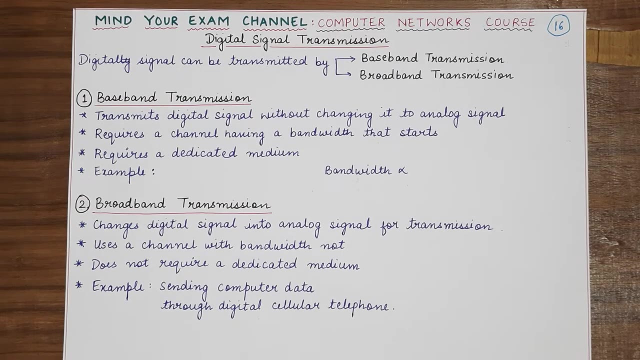 Hello students, welcome back to my channel. In this video we will be doing two types of digital signal transmission. So first is the baseband transmission and the second is the broadband transmission. So in the previous video we have learned that information in the form of 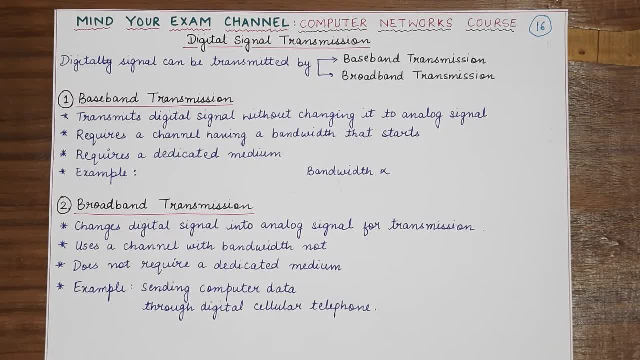 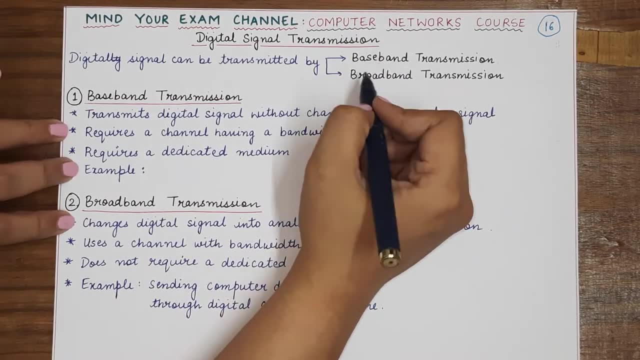 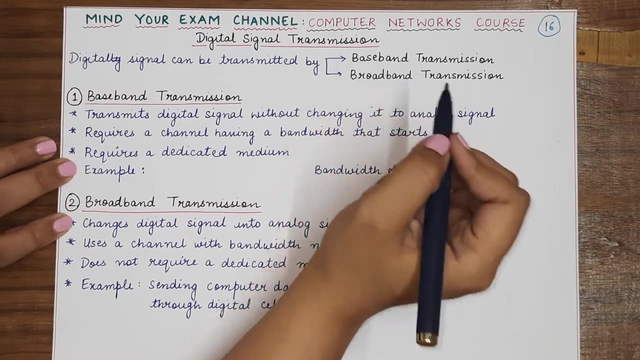 signals can be transmitted either in the form of analog signals or in the form of digital signals. Now, digital signal transmission can be done either using baseband transmission or broadband transmission. Okay, now let's understand what are each of these. In baseband transmission we 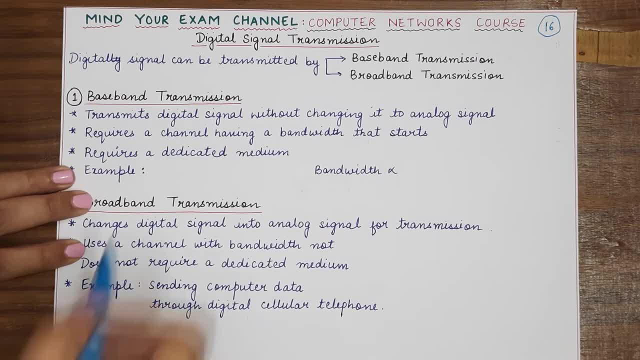 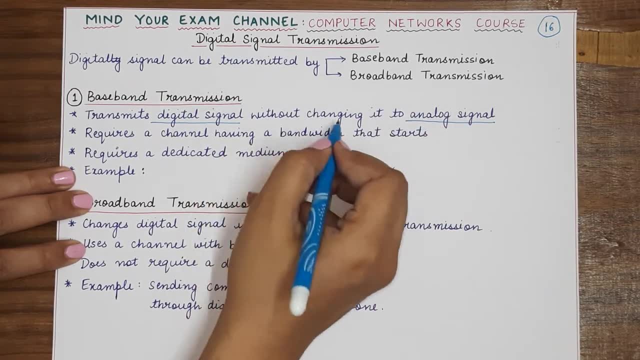 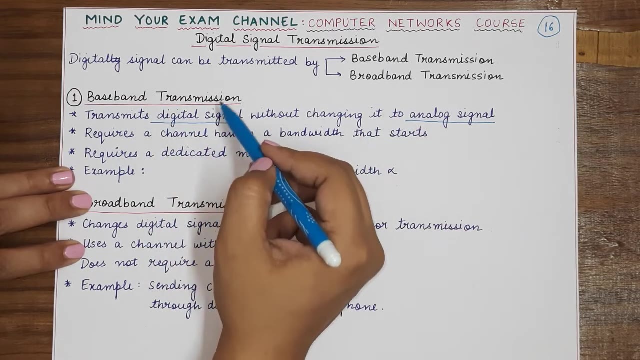 basically are transmitting a digital signal, but we are not changing this digital signal into an analog signal. Okay, so, without changing the digital signal in its original form, we are sending it during. So we are sending baseband transmission through the transmission channel or the communication link. 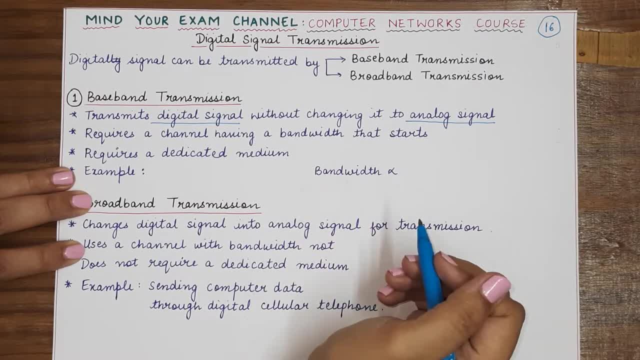 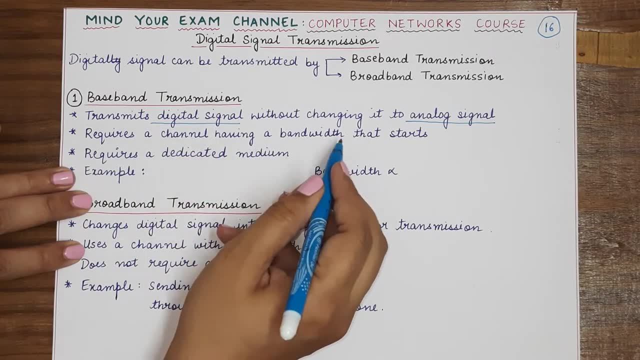 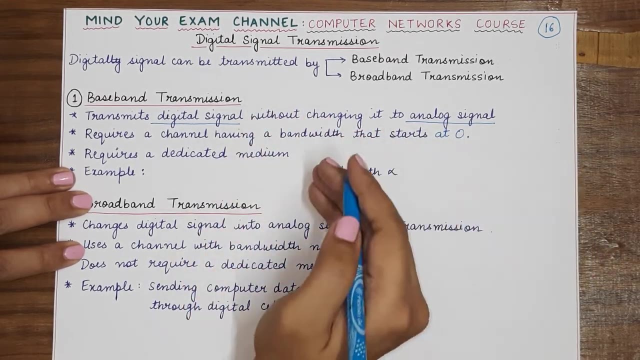 or the physical media that you are using for transmission. Okay now, a baseband transmission requires a channel that has a bandwidth which starts at zero. Okay, so the bandwidth must be starting at zero. The range of frequencies is known as the bandwidth and the channel needed. 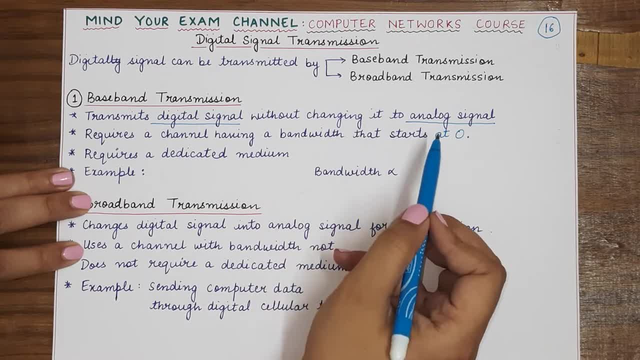 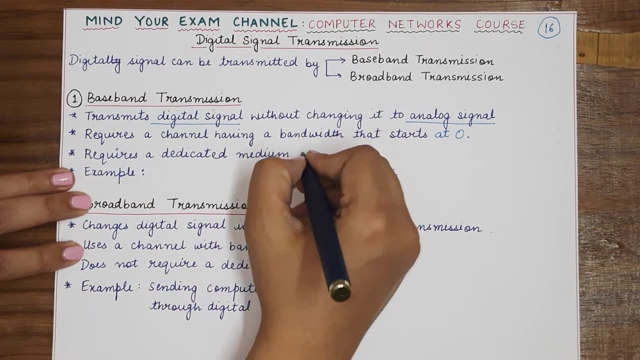 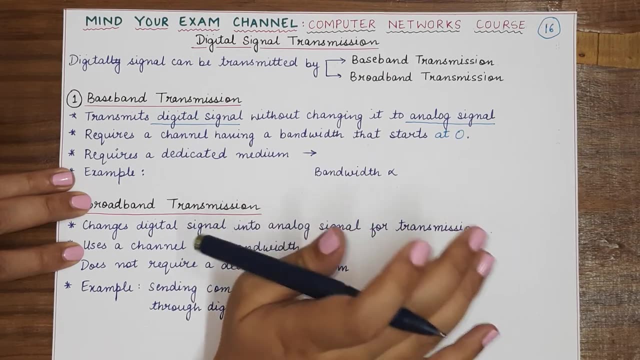 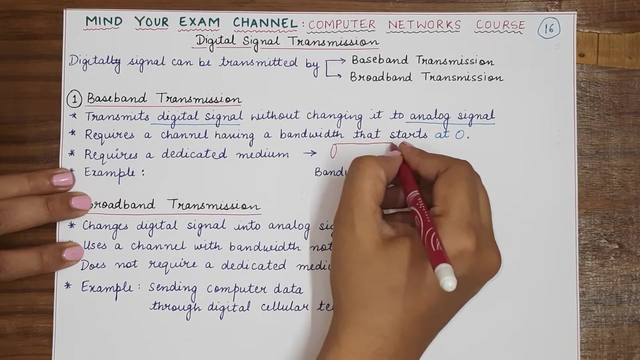 for baseband transmission Should have a bandwidth that starts at zero. Also, baseband transmission requires a dedicated medium. This means that when signal is propagating, only one frequency will be propagating through that. Multiple frequencies cannot be sent through the channel. That means if communication is happening. 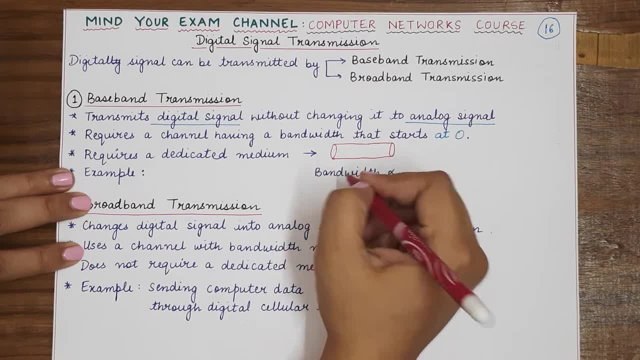 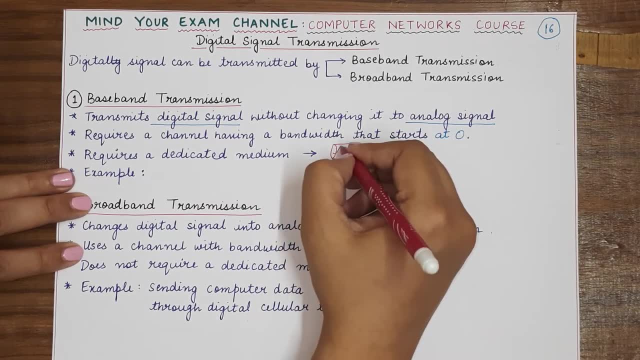 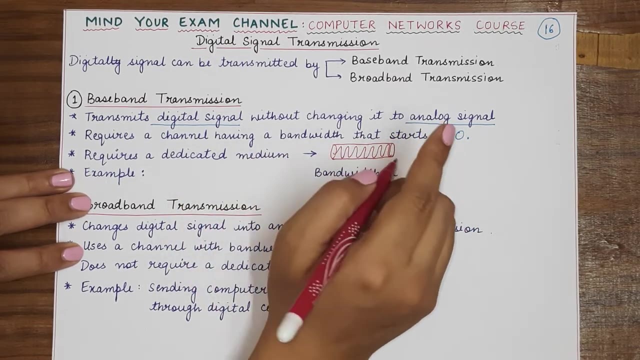 between a particular sender A and receiver B and if this channel is not sending a particular signal, the signal is shared by other people also, Then at a time, only one signal will be sent at any given time. This medium will behave as a dedicated medium and it will not be shared. 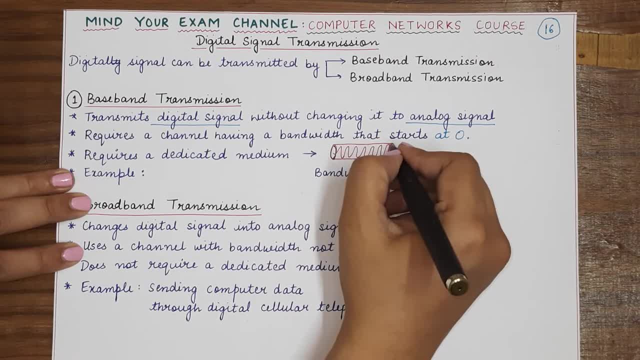 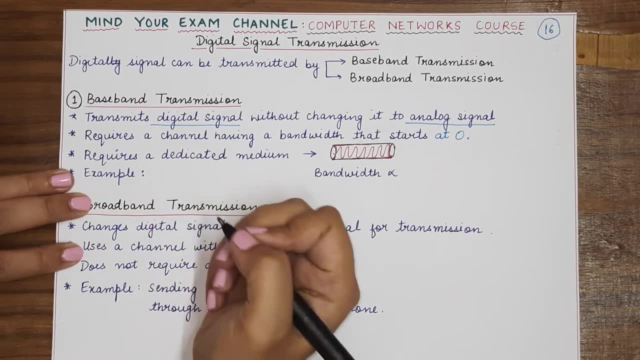 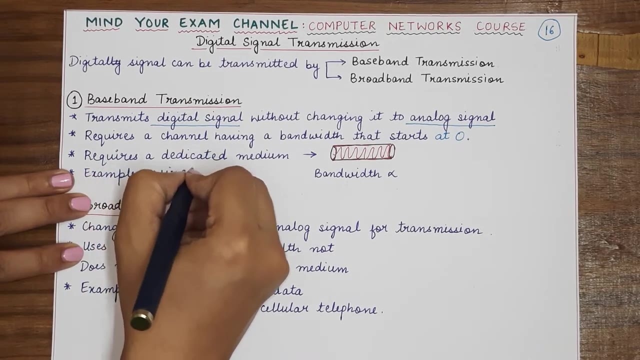 So these are the requirements for baseband transmission. Okay now the example of baseband transmission is the wired LANs that we use in our homes. They are applicable or they are used for at different places in our professional lives also. So wired local area networks use baseband. 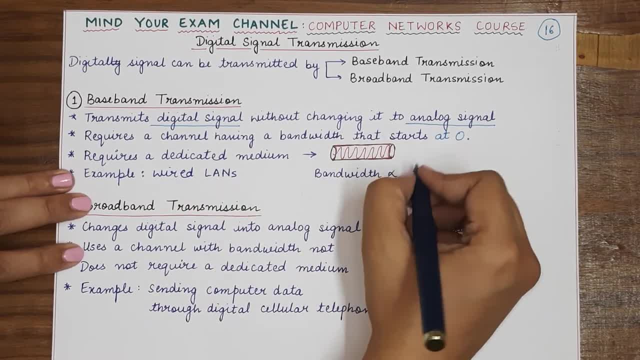 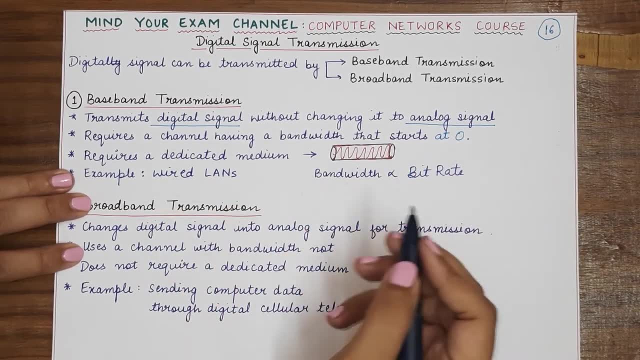 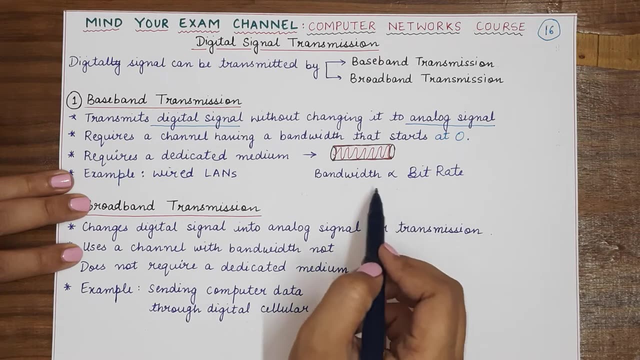 transmission and in baseband transmission the bandwidth is directly proportional to the bit rate. that means if you want to increase the number of bits that you want to send, that means if you want to increase the bit rate, you will have to increase the speed of transmission also. you will. 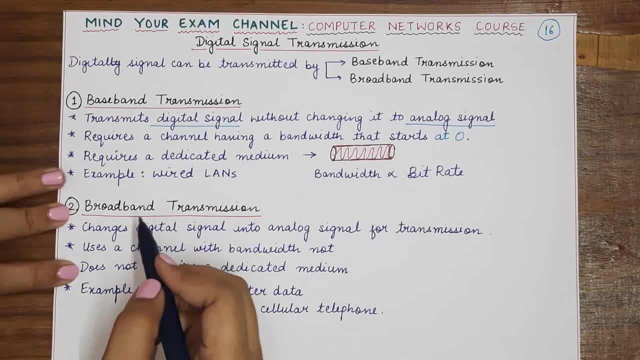 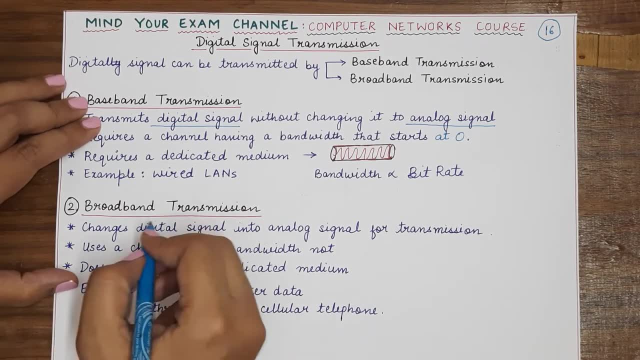 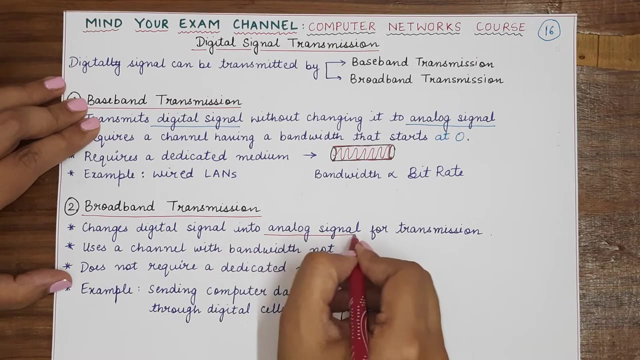 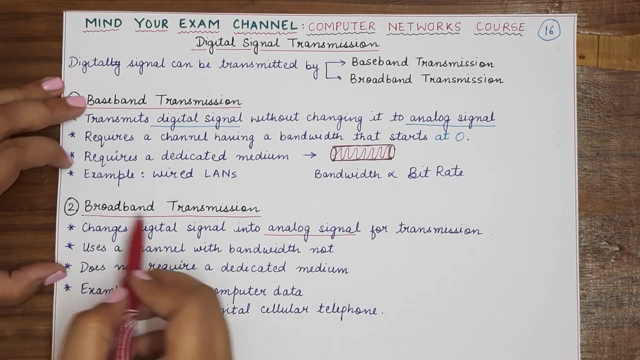 have to increase the bandwidth also. Now coming to the second kind: broadband transmission. Now, in broadband transmission, to transmit digital signal, this signal is first converted into an analog signal and this analog signal is then sent over the transmission link. Now, in case of broadband transmission, the channel that is used for transmission. 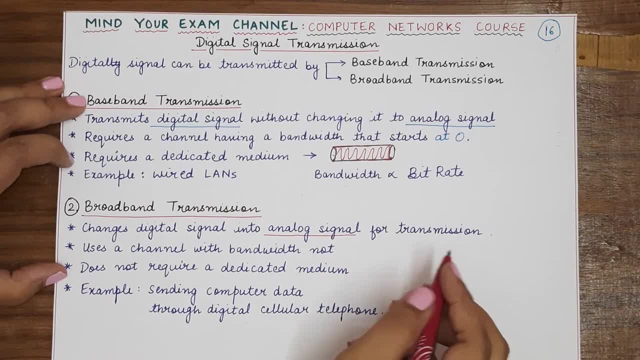 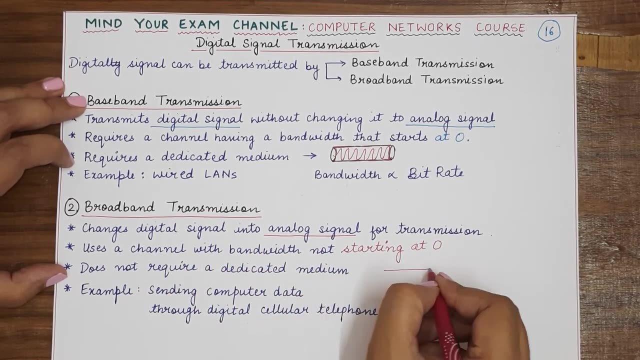 may not have a bandwidth that starts at zero. So, with bandwidth not starting at zero, and also the channel may not be dedicated, The channel might be shared by multiple parties and multiple signals might be transmitted through the channel by dividing it logically into separate parts. 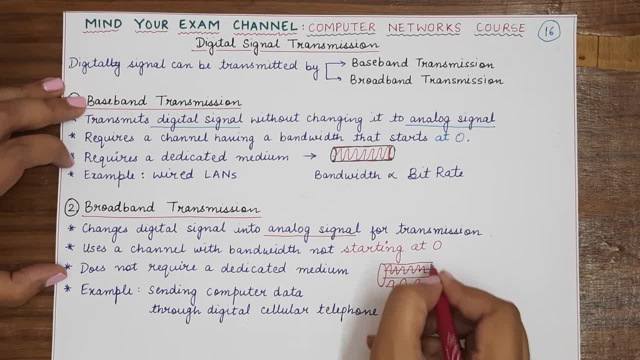 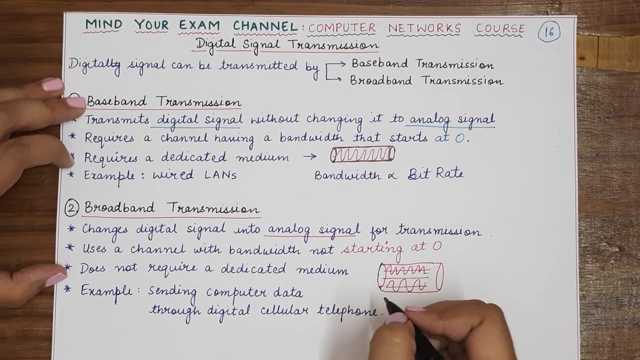 So the link through which, or the physical medium through which communication is happening can be shared in the case of broadband transmission, And the most common example that uses broadband transmission is the digital cellular telephone, which is used to send computer data. Okay, so these were the two kinds of digital transmission that 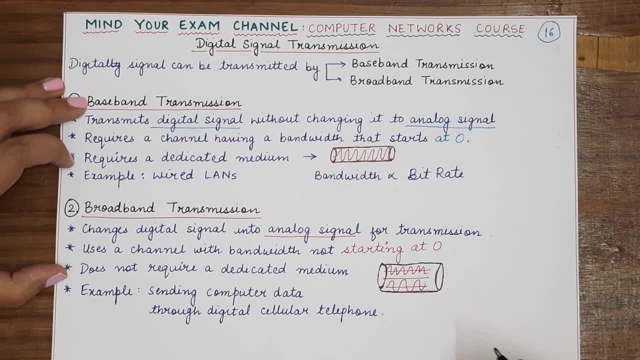 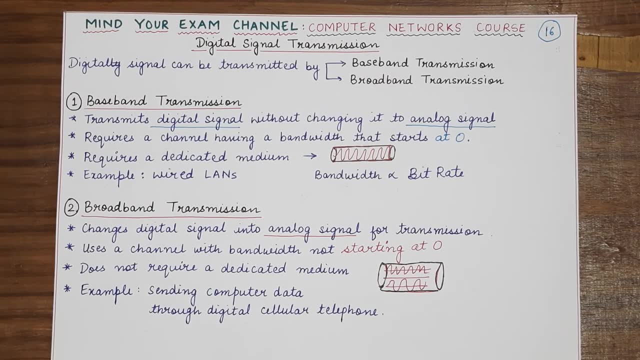 can be used for transmitting digital data. One is the broadband transmission and the other is the baseband transmission. So that's all for today. Thank you for watching, Till we meet in the next video. mind your exam.